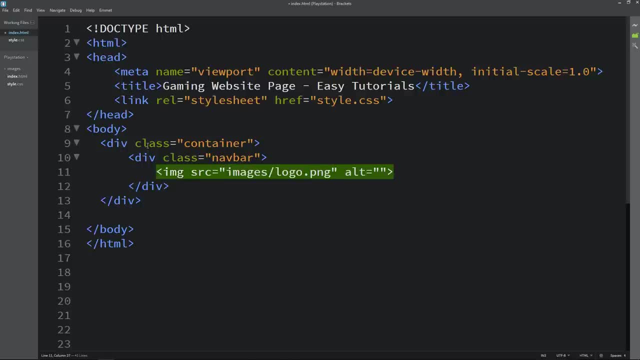 div with the class name navbar. In this navbar I will add one image and let's add one class name logo. Let me duplicate it and we will add the another icon, which is for menu and class name menu icon. Now we have two icons here. Between these images we will add one tag nav where we 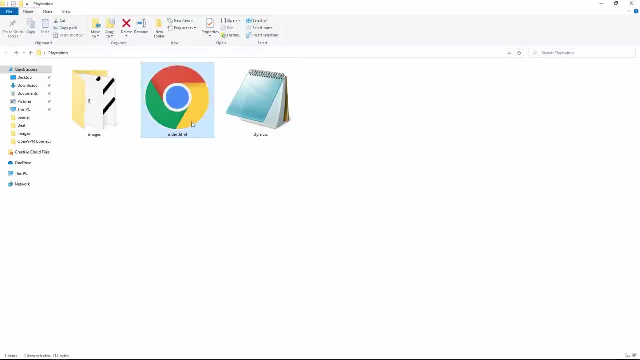 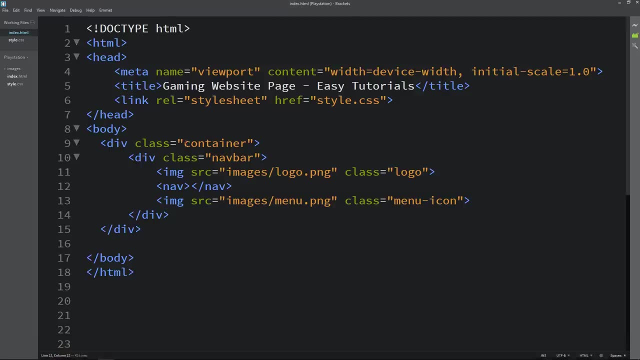 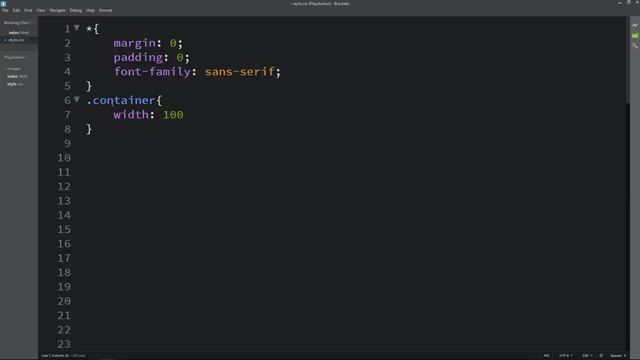 will add the navigation links. Now I will open my HTML file with Google Chrome so that you can see one menu icon on this web page. Let's come back in the HTML file, and here we will copy this class name container. Write it here in this CSS file. For this one we will add the CSS properties like: 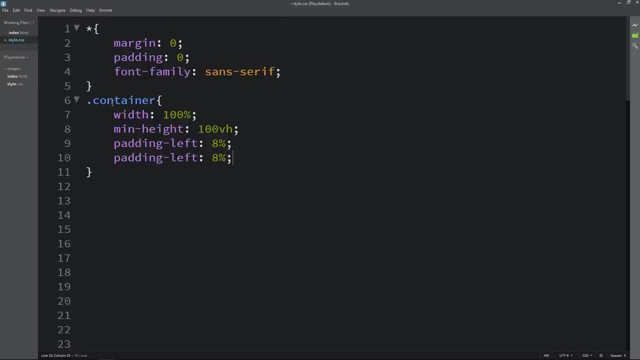 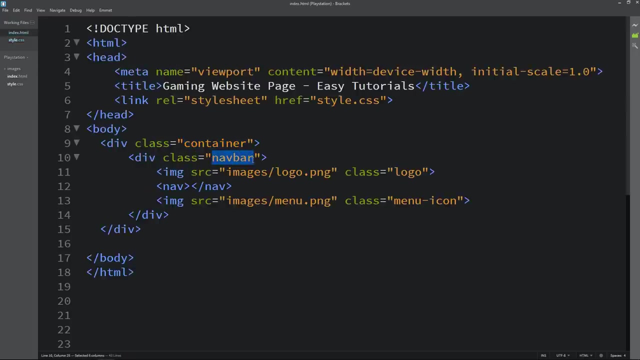 width, min height, then padding from the left side and right side Box sizing will be border box and overflow hidden. Now you can see summer space from the left side. Let's copy the class name navbar, Write it here in the CSS file. For this one we will set the width. 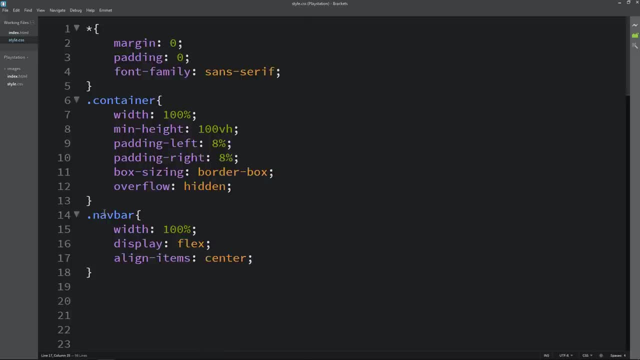 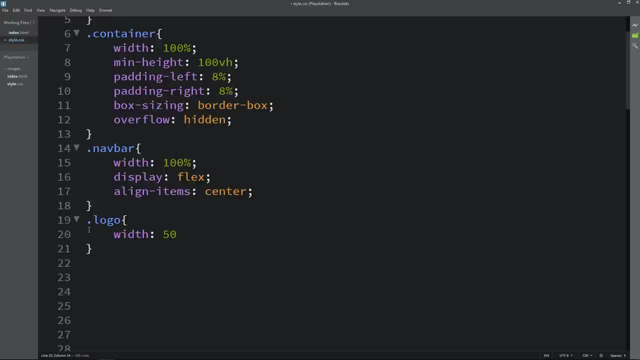 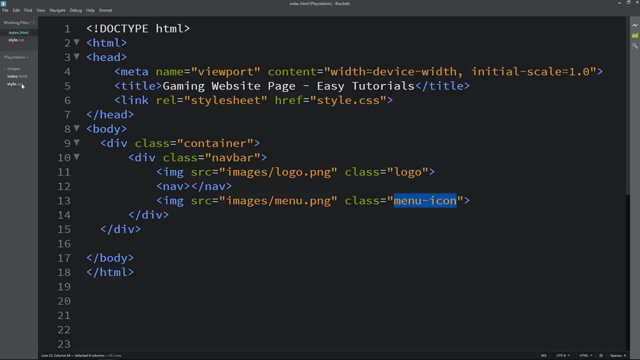 100% and display will be flex and align items center. Let's copy the class name logo. For this logo, we will add width, It will be 50 pixel and cursor will be pointer. Then margin: 30 pixel and zero. Let's copy the class name for the menu icon, Write it here and here we will add width. 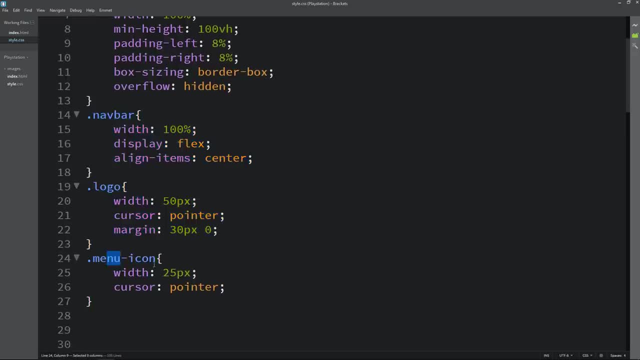 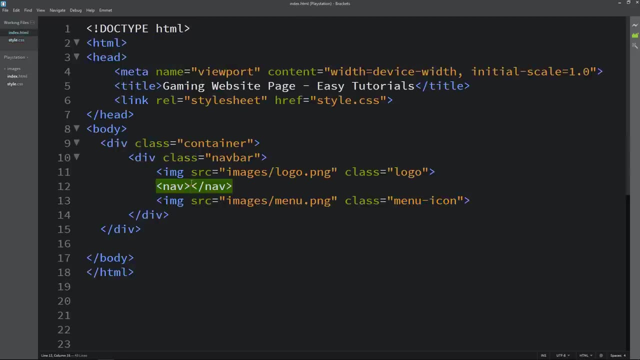 and cursor will be pointer. Let's copy the class name logo. For this logo we will add width and cursor pointer. So after adding this, let's refresh the web page and now you can see a small logo and icon. Let's come back in the HTML file and in this snap we will add some links. So here I am adding. 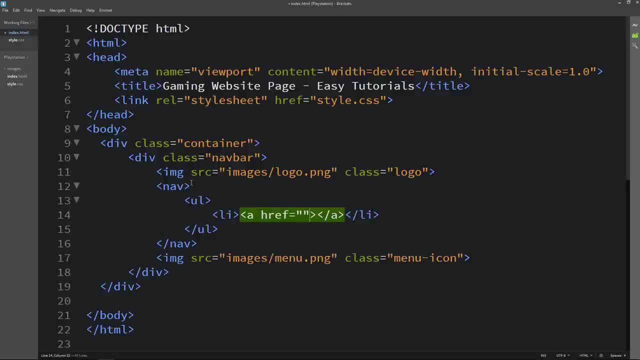 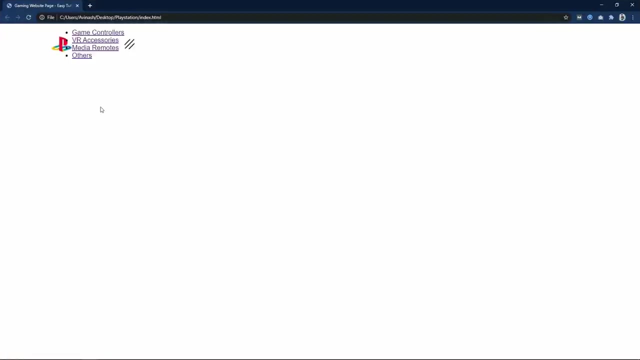 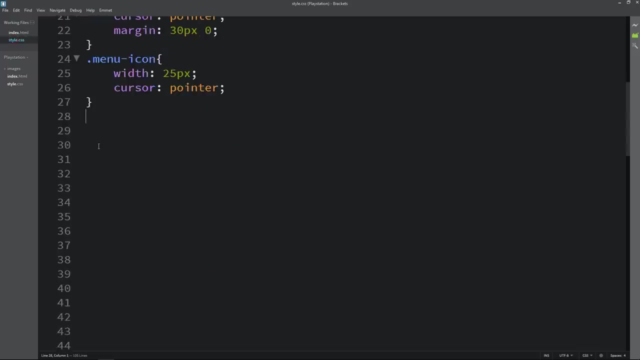 ul and li, Then anchor tag and here we will write the text. So this is the first menu. Let's duplicate it and we will change the text. So now we have four links here. You can see that. we have four links here. You can see this on the web page. Now just copy this snap. Write it here. For this one write: 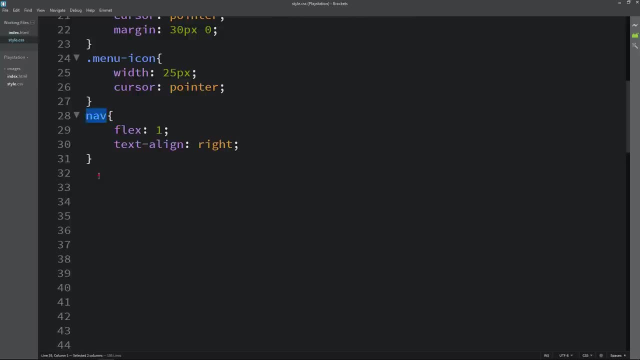 the flex one and text align right. Let's copy it again. then write ul and li For this list. I will write list style none and display inline block and margin from the right side. Now it is coming in the right side. Next we have to add CSS for the anchor tag, So just copy again. Write a Here we will. 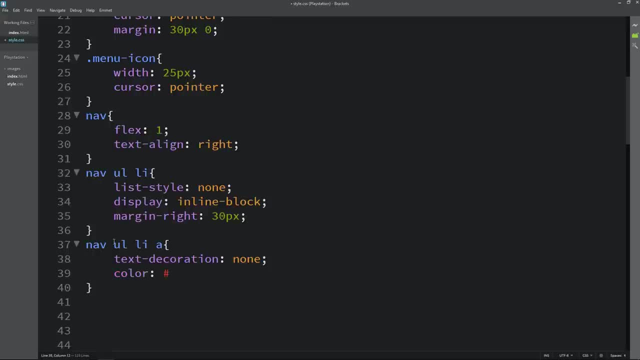 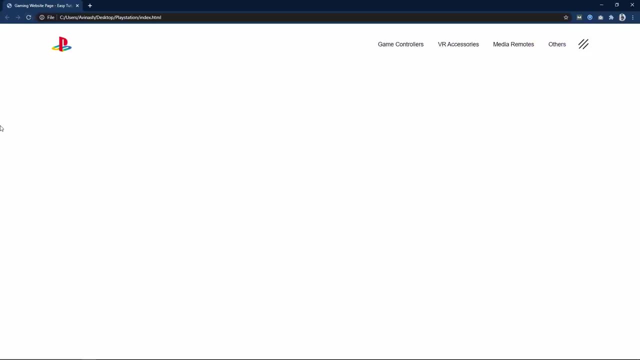 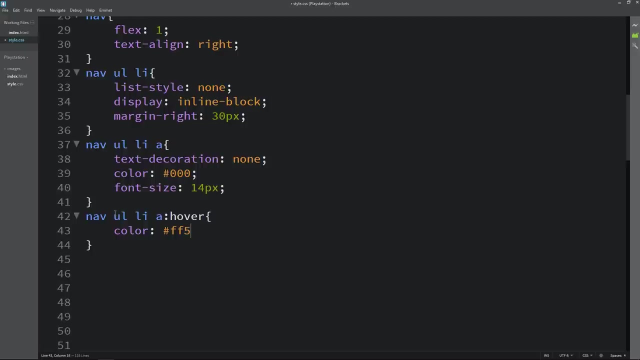 write text decoration none, and we will change the color. and for the anchor tag we will write text font size. So now this menu is looking good. Next we have to add hover effect on this menu. So just copy again: Write hover, and here we will change the color. That's it Now. you can see if I take. 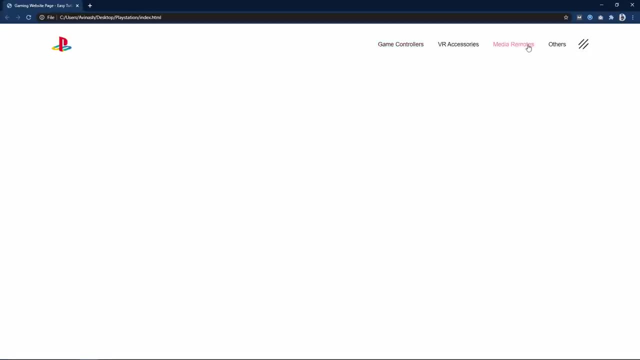 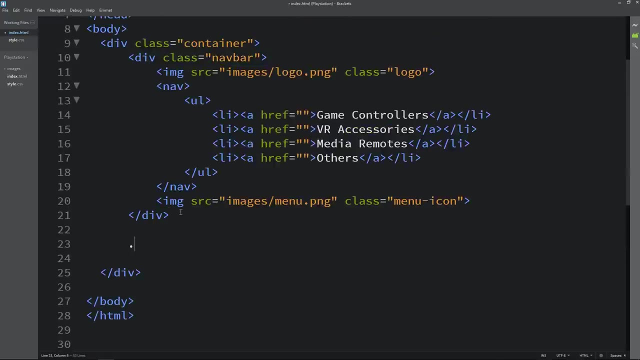 cursor over this menu, you can see the color is changing. After creating this navigation bar, we will add some content on this web page. So just come back. and after this nav bar here we will create another div with the class name row, and in this row we will add some content. So just come. 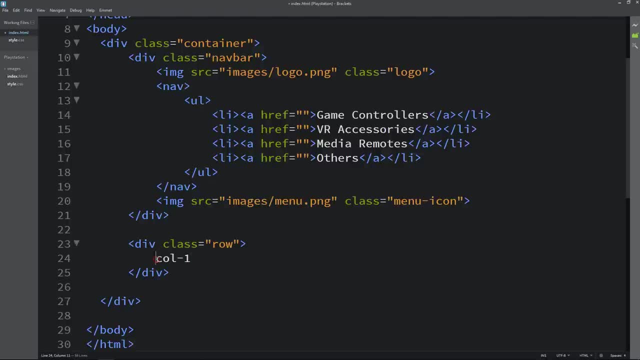 back, and after this nav bar here we will create another div with the class name row and in this row we will add some content. So just come back, and after this nav bar, here we will add some content. So let's create one more div with the class name Call one. Let's duplicate it and it will be call. 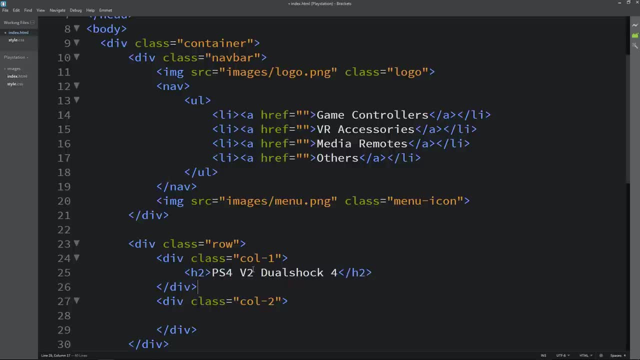 two. So we have two columns Now. in the first one we will add one title in h2.. So this is the title. Let me add one more title in h3.. So this is the h3 text. Let me add one more text in p tag. So this: 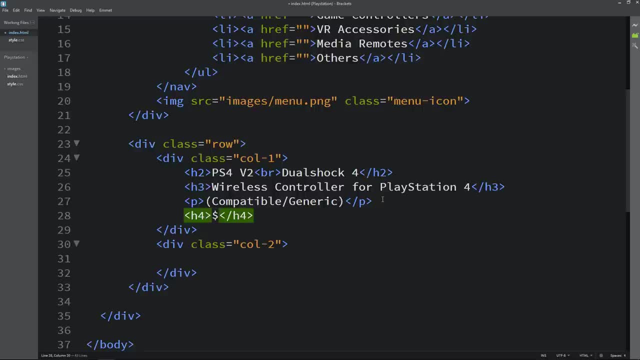 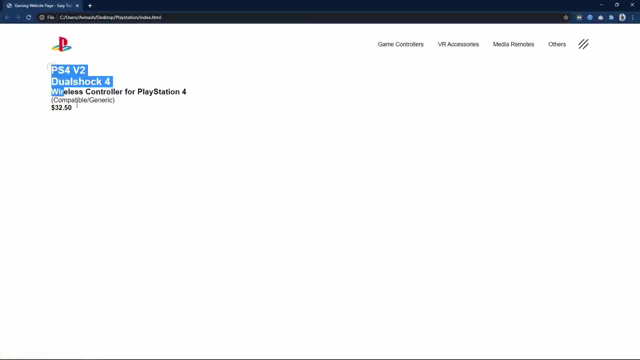 is the small text. After that I'll write price in h4 tag. So after adding all these content, reload the web page and you can see all this text on the web page now. if you have to design it, so just copy the class name row, write it here in the css file and for this row we will set. 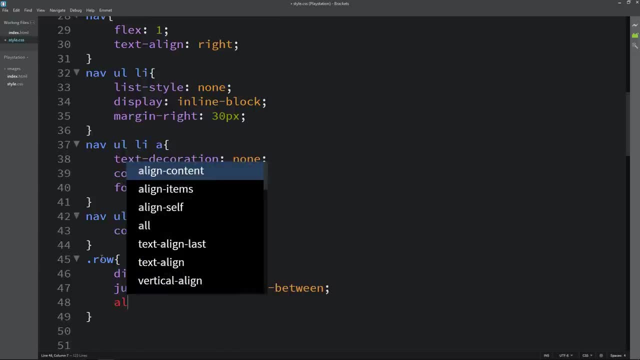 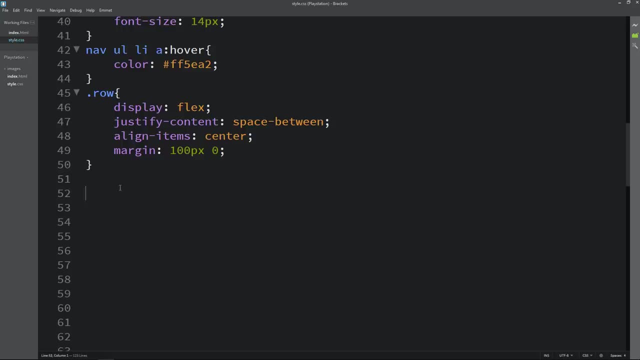 display flex and justify content. space between align items will be center and margin: 100, pixel 0.. let's copy the class name, call 1, write it here and here we will write: flex, basis 40 and position relative, then margin from the left side. now it is coming here. now let's copy again, then write: 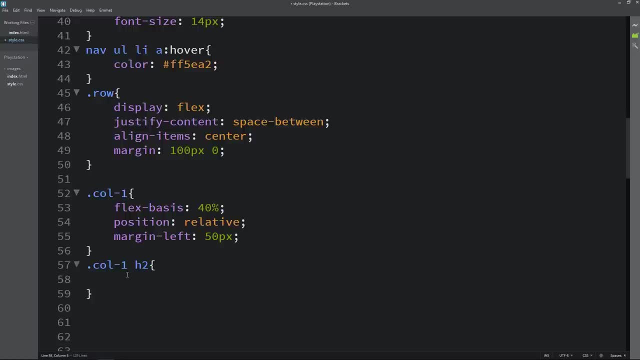 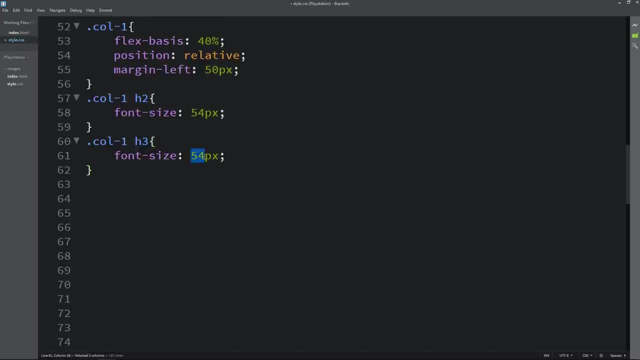 h2 for the text. and for this h2 we will write font size. we will increase the font size. let's duplicate it and it will be h3. and here we will write 30 pixel, then color, this color code, and font weight, then margin. let's copy it again. 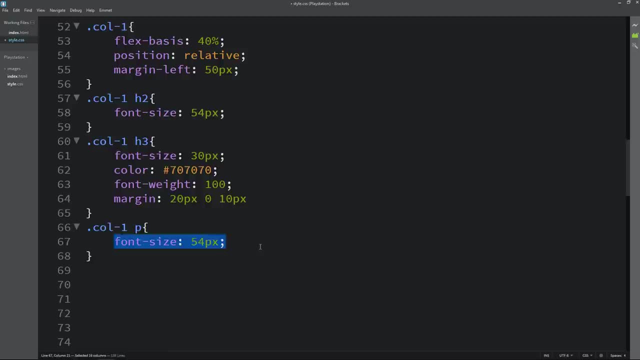 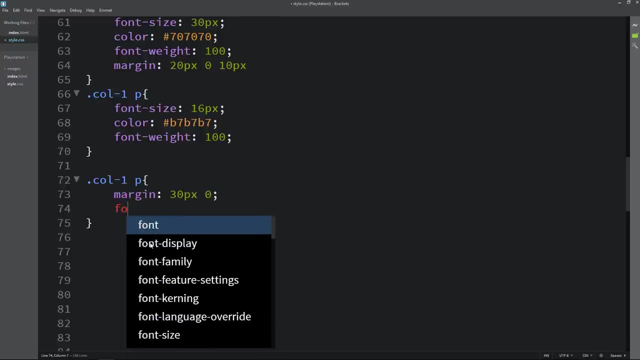 write it here, and here we will write p for the text. here we will change the font size and color, and font weight will be 100. now you can see it is looking like this. next we have to write css for h4, so just copy again. then write h4 and here we will write margin: 30 pixel and 0, then font size: 20 pixel. 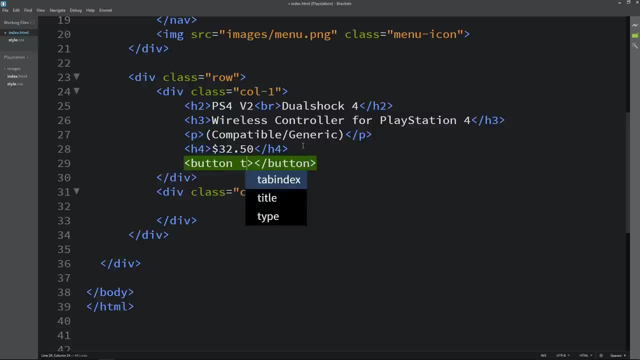 now let's come back in the html file. here we will add one button. so i'm adding button, type button and by now it is text, and this button will add one icon also. so i'm adding img, then src file path, which is arrowpng. after adding this button, 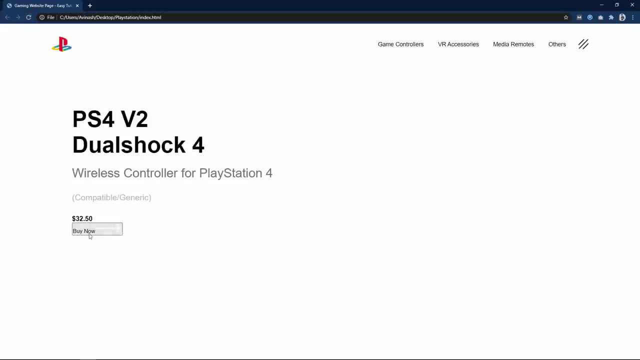 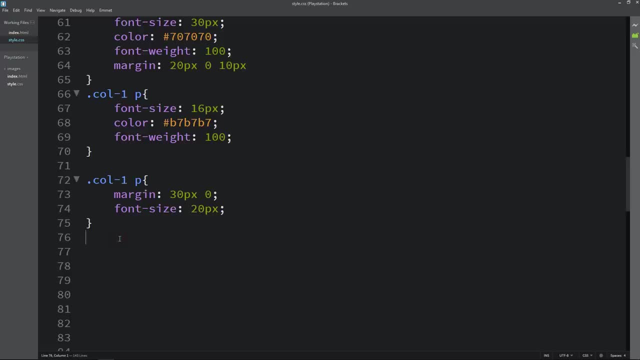 let's refresh the webpage. on this webpage you can see this button with an icon. now just copy this button, write it here in the css file. here we will write: width: 140 pixel and border 0 and padding 12 pixel and 10 pixel. outline will be none and color white. then background: linear gradient, and here we will write: 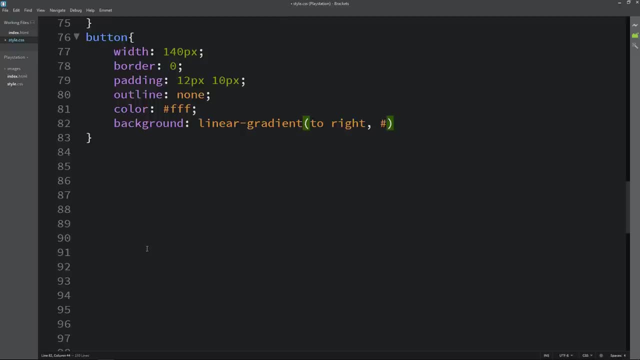 to right and we will add two color code. so this is the color code first one and this is the second one. outline will be none and color white, then background, linear gradient, and here we will write two right and we will add two color code. so this is the color code first one and this is the second one. outline will be none and color white, then background, linear gradient, and here we will write two right and we will add two color code. so this is the color code, first one and this is the second one. outline will be none and color white, then background, linear gradient, and here we will write two right and we will add two color code. so this is the color code, first one and this is the second one. 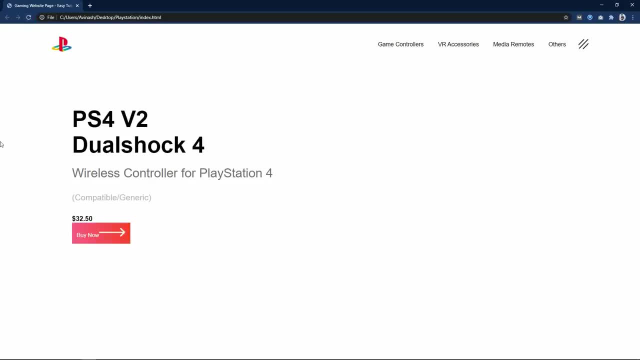 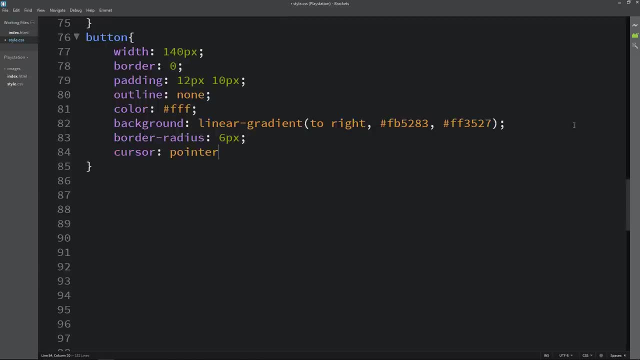 after adding this, you can see we have the gradient color in the background. next we will add border radius and cursor pointer. now it is looking like this. let's copy this button, then write img, and for this one we will set the width: 30 pixel. and now you can see it is looking like this: 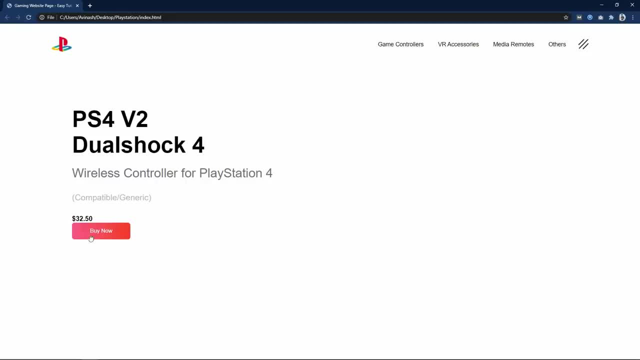 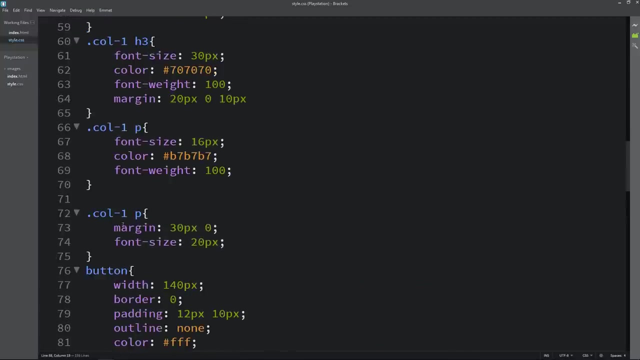 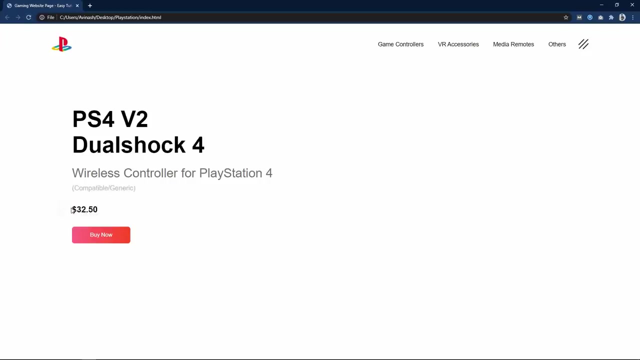 here we will add display none, so the icon will be hidden, and when we will hover this button then the icon will be visible. you can see we have no space here. let me check. so here we have one mistake: instead of this p we will write h4. so now we have some space here before this button. so let's come back in the css file. 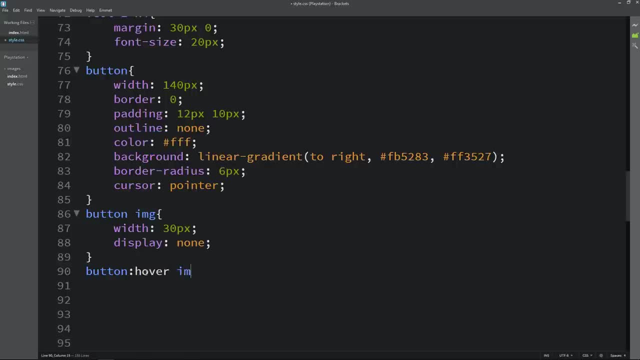 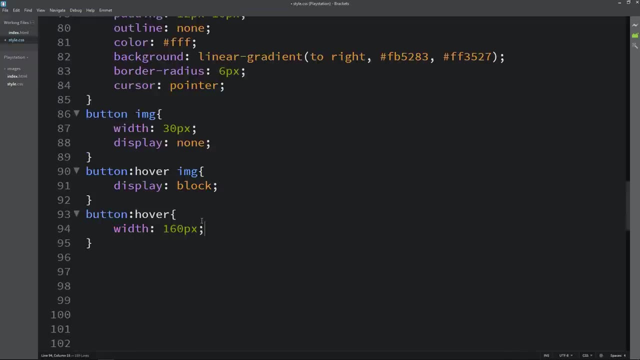 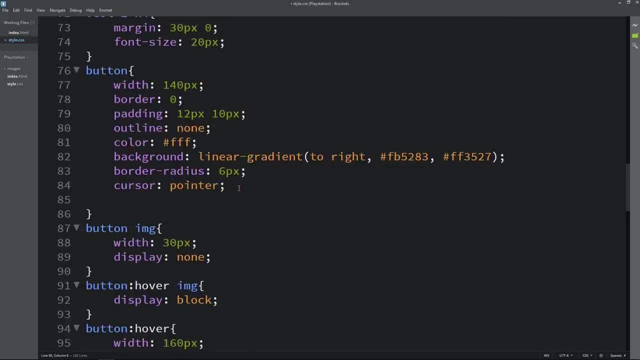 just copy this button, then write hover and img. here we will write display block, so it will be visible. let's copy it again. then write width: 160 pixel display flex and align item center: justify content. will be space between. here we will write transition: width: 0.5 seconds. 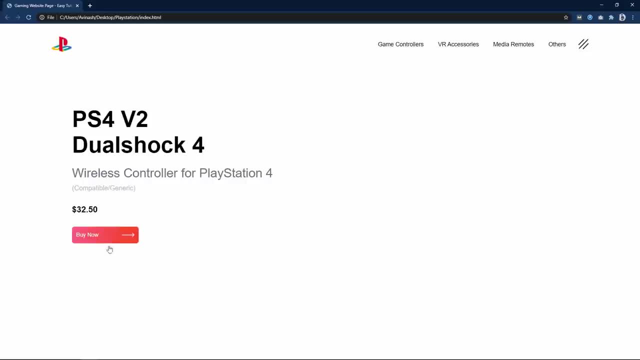 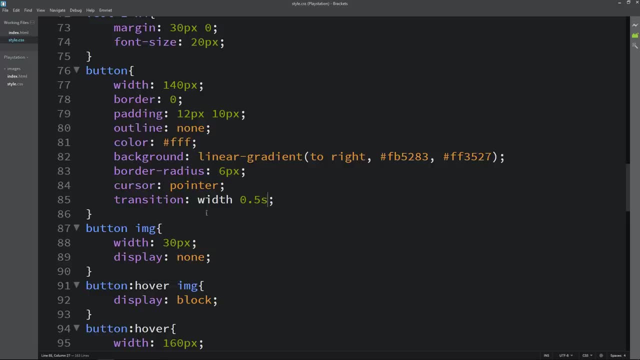 now you can see, if i take cursor over this button, its width is increasing and it will display one icon in this button. after that we will add one vertical line in the left side. so just come back. come back, copy this class name col1, then write after: here we will add. 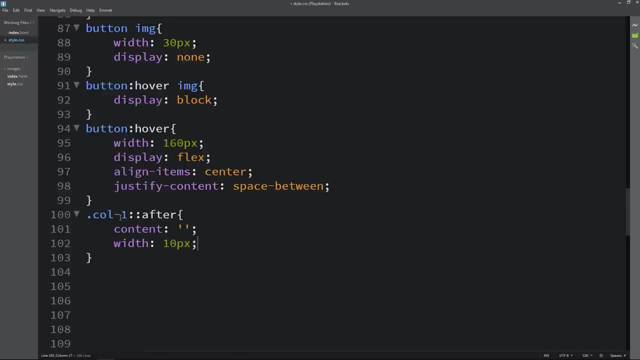 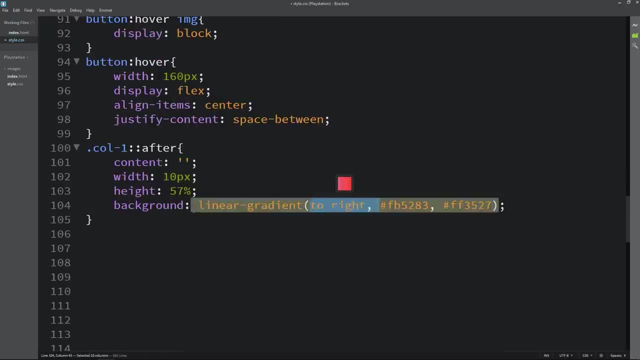 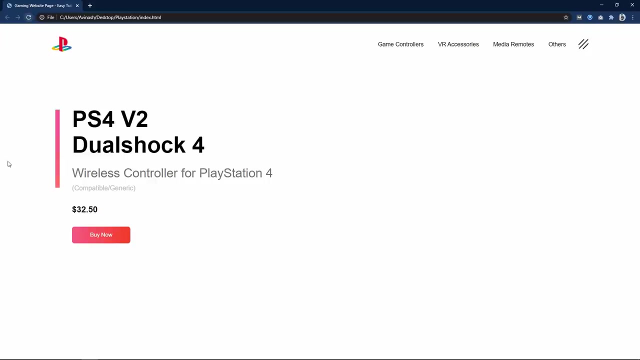 content: empty. width: 10 pixel and height 57%. background will be linear gradient color. let me copy this one here. we will change the color code. after that we'll write position: absolute left minus 40 pixel and top: 8 pixel. now you can see one vertical line in the left side. after that we will add some content in the 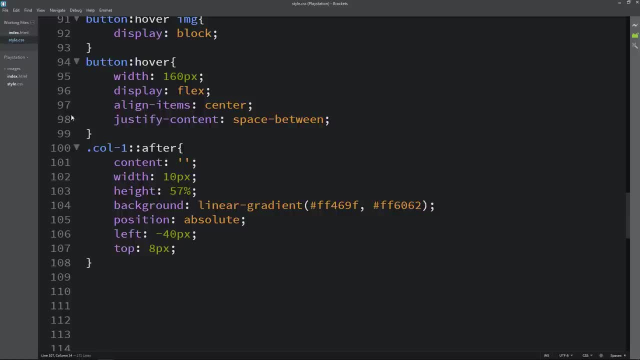 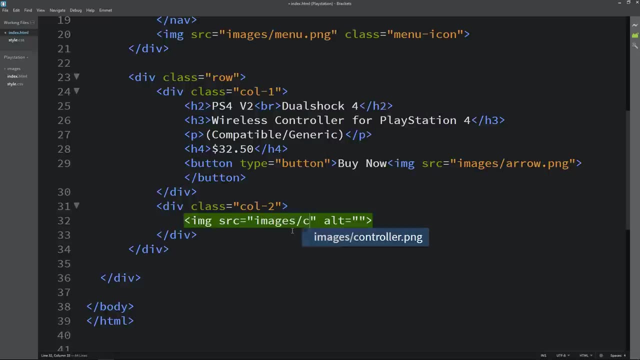 right column, which is column 2. so let's come back in the HTML file and here we will add one image. so I am adding IMG tag, then file path and one class name. so let me add the class name controller. let's copy this one here. we will add a class name and a class name. so let me add a class name. 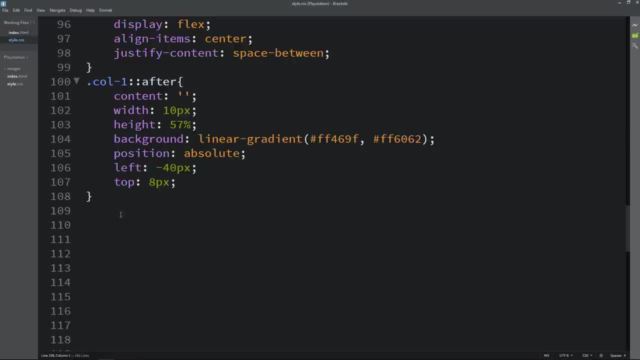 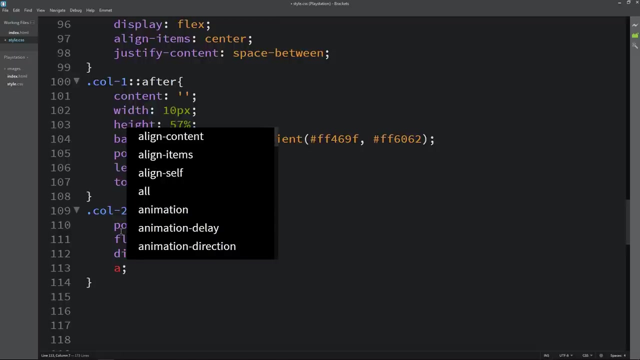 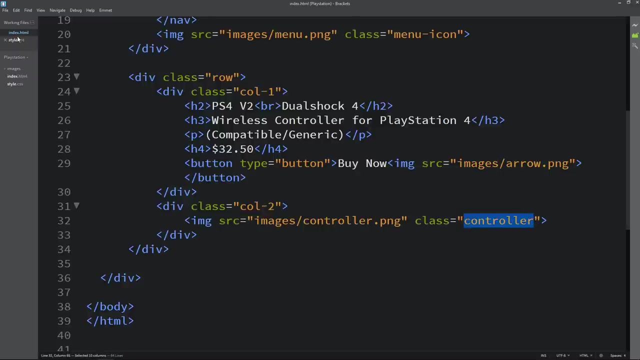 right now. you can see this controller is very weak, so just come back in the CSS file, write this class name col2. then here we will add position: relative flex basis 60% and display will be flex align items center. copy this class name controller, write it here. before that I will add the class name col2 for this one. 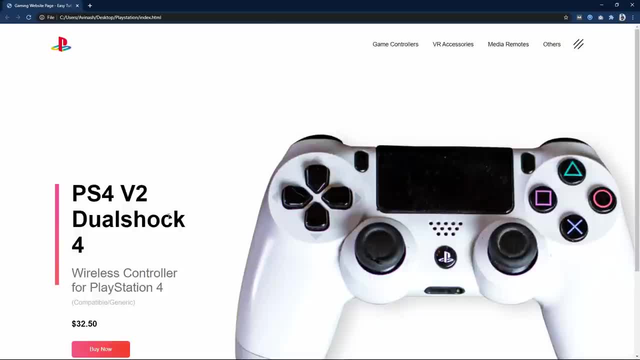 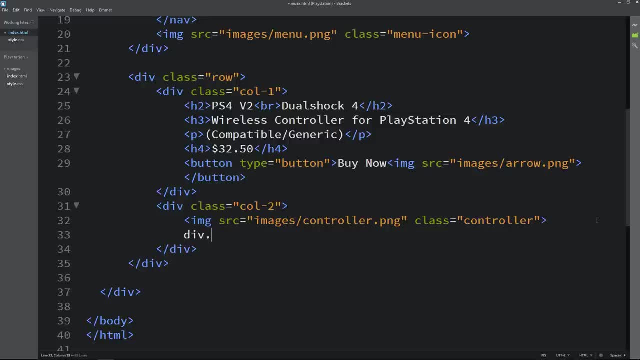 we will set the width. it will be 90%. now you can see small controller image here. let's come back and here in the HTML file we will create one tip with the class name color box. let's copy this class name. write it here in the CSS file. 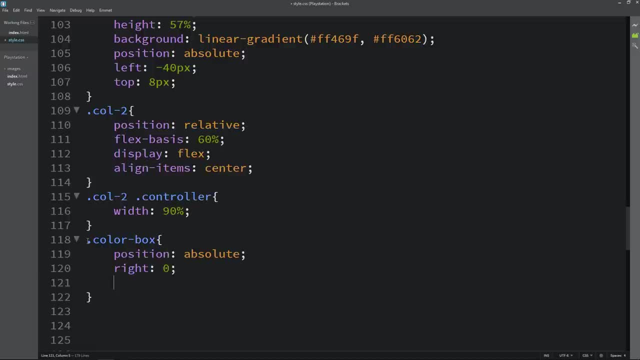 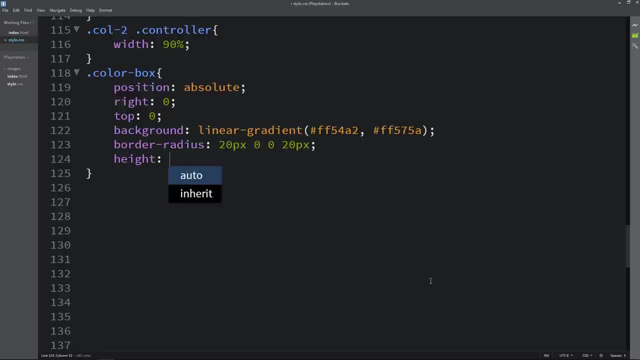 and for this one we will write position absolute and write 0 and top 0, then background it will be linear gradient color- you can keep the same color- and then border radius: 20 pixels: 0, 0 and 20 pixel. height: 100% and width: 80% z-index. 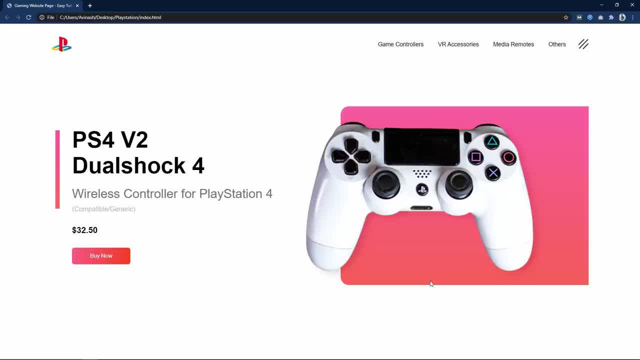 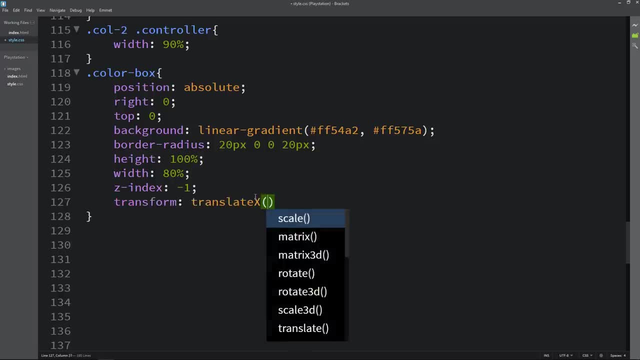 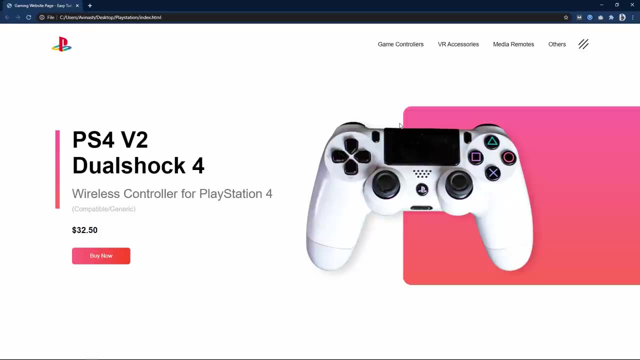 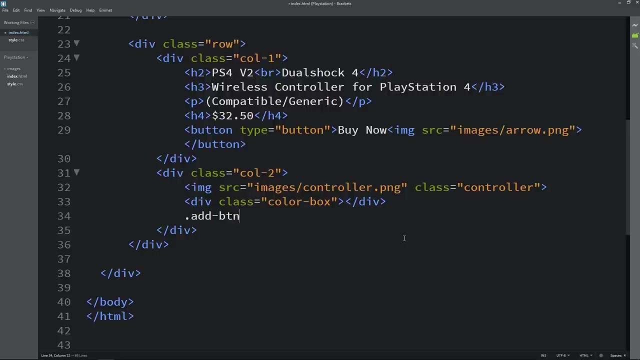 minus 1. now you can see one colored in the background. now we have to move this color box in the right side. for that, here we will add transform translate X 150 pixel. so now it will be on the right side. that's it, let's come back. and after this tip we will add one more tip with the class. 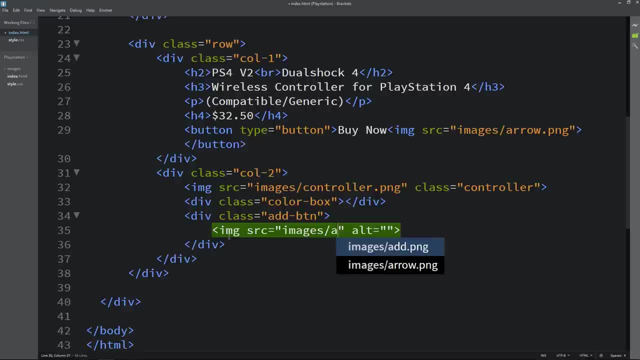 name, add BTN, and here we will add one IMG and the file path. after that we will write one, a small text- for that I am using P tag and a small- and the text is add to cart. after adding this, let's refresh the web page and you can see. 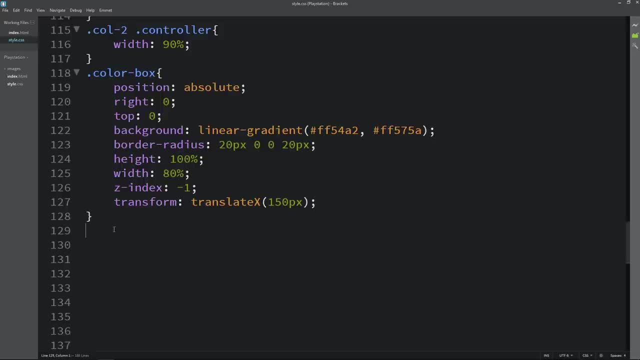 this big icon and one small text. let me copy the class name: add BTN. write it here in the CSS file, then write IMG. for this image we will set the width, 35 pixel and margin from the bottom. now you can see image size is good, let's come. 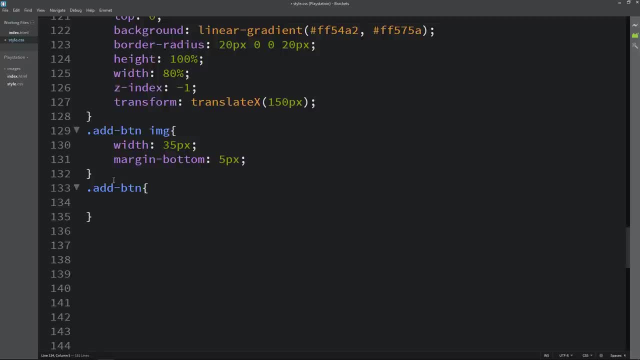 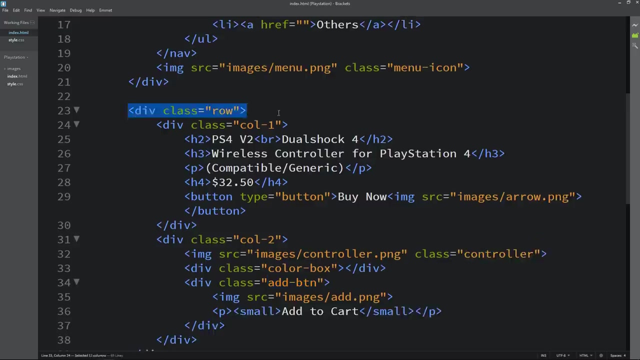 back and copy this class name again and here we will write text: align: center and color white cursor will be pointer. now it looks good. after that I'll add some social media icons at the bottoms. so after closing this row dip, we will create one another to be the class name. social links: here we will add social. 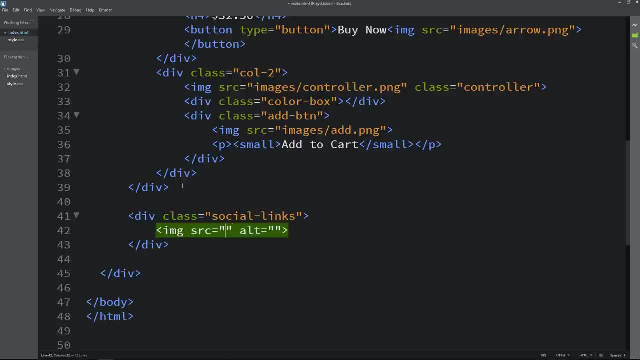 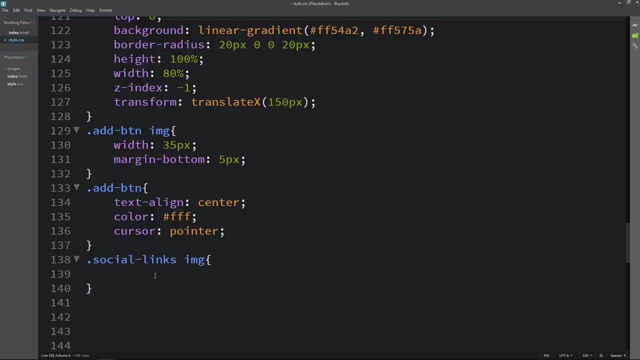 media icons. so I am using IMG tag, then source, then file path, duplicate it and change the file name. so we have three icons. let's copy this class name, write it here in the CSS file and here we will add IMG height. it will be 13 pixel and 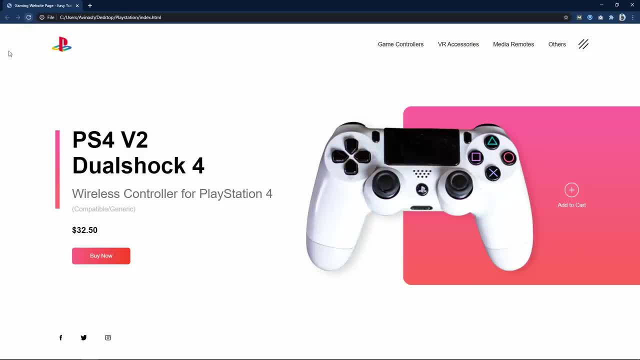 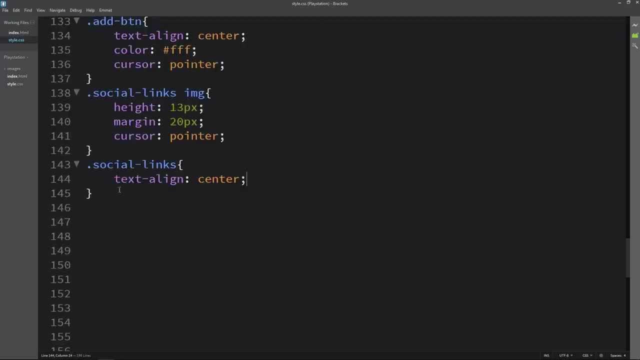 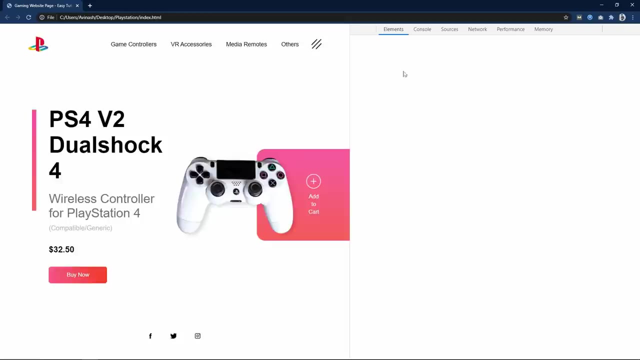 margin: 20 pixel and cursor pointer. now you can see these icons in the left side, so we have to move it in the center. so just copy again. then write text: align Center. that's it. now you can see these icons in the center. next we will change the screen size so that you can see this. 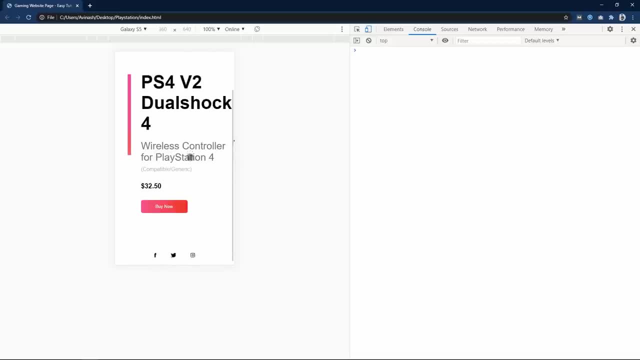 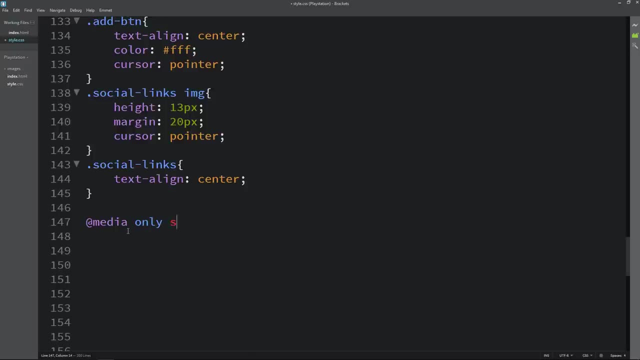 page is not responsive right now, so we have to add media queries to make this web page responsive. so come back in the CSS file. here we will add media only screen and max width: 700 pixel. now, whatever CSS properties we will write in this media query, that will be. 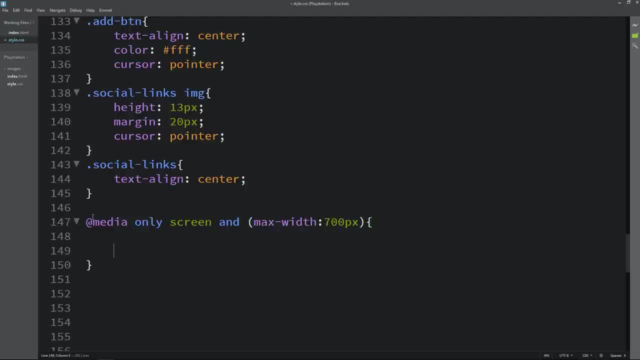 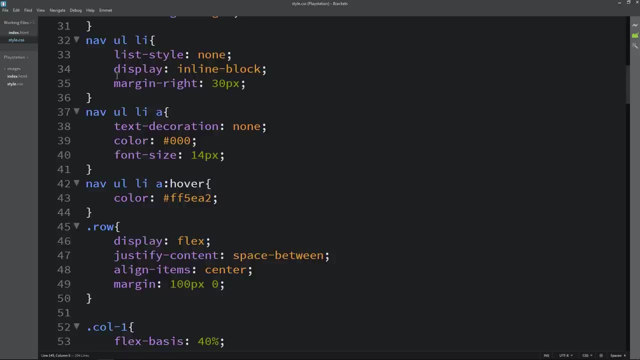 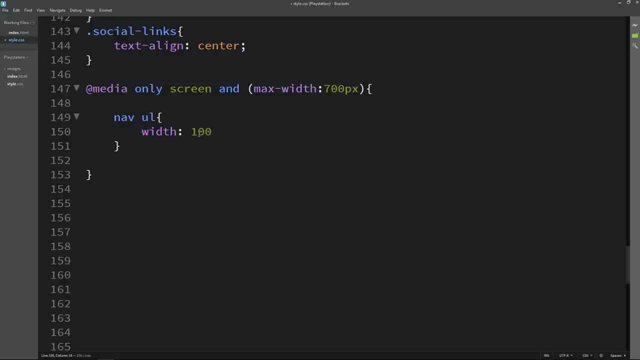 applicable for device whose width is less than 700 pixel. so first we have to write the CSS for this navigation menu. so come back in the CSS file. here you can see we have this nav and ul. so let me add this one nav ul: width 100 percent and background: it will be linear gradient. let me copy from here. that's it. 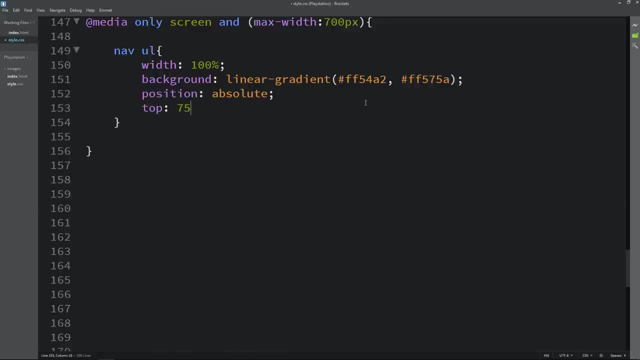 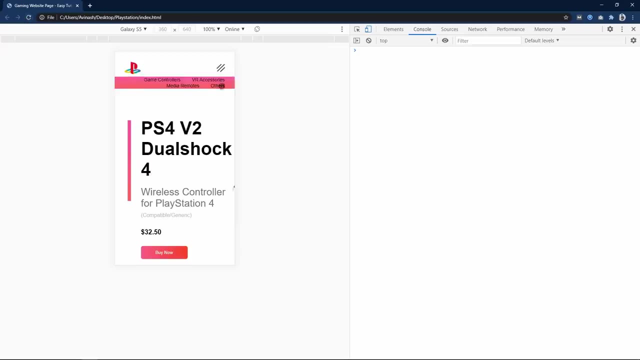 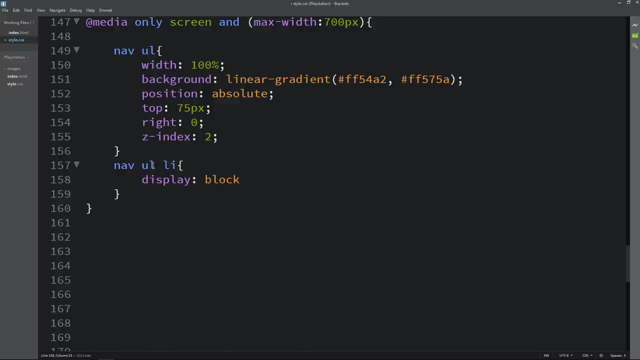 then write position absolute and top- it will be 75 pixel- and write 0, z-index 2. after adding this, you can see it is coming like this. let's come back and just copy again. then write li- it will be display block and we will add some margin from the top and margin from bottom. 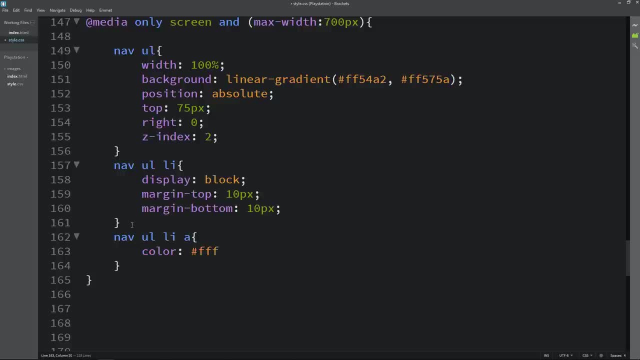 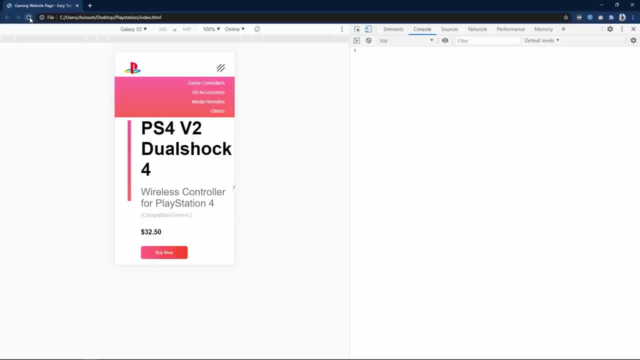 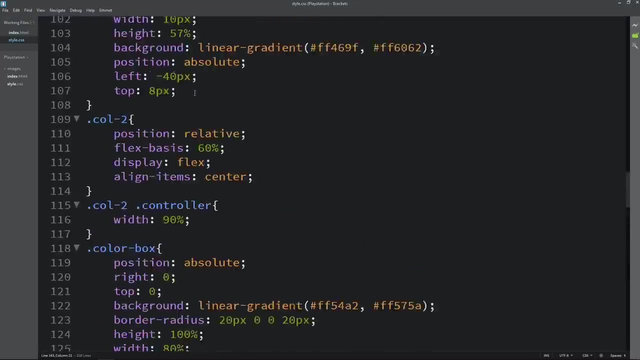 let's copy it again. then write a and we will change the color. now it is coming vertically. right now you can see this icon is visible on fuller screen also and a smaller screen also. so we have to hide this icon on the larger screen. for that we will come back in. 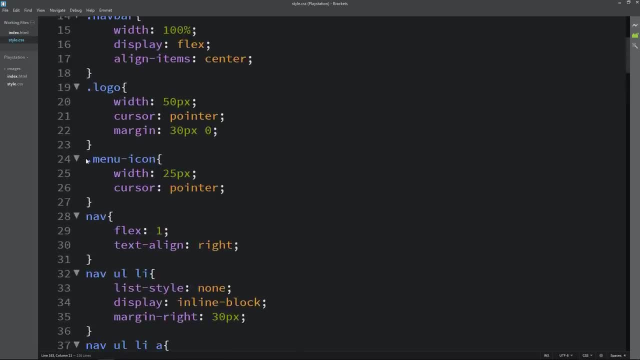 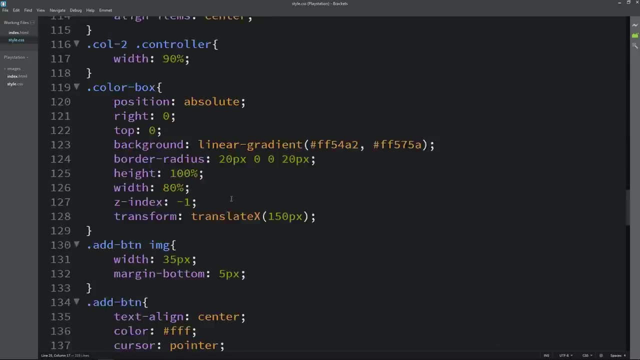 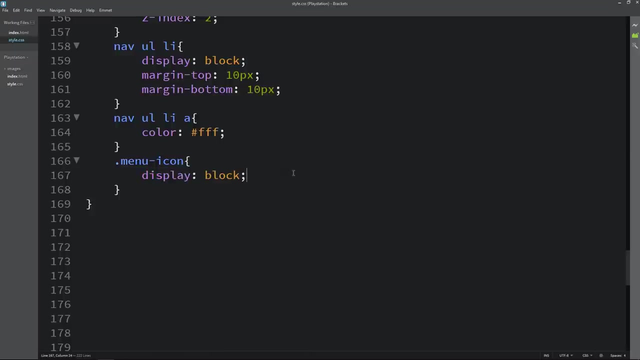 the CSS file and here we have written menu icon. so let's add display none. now just copy this menu icon, come to the media query and in this media query we will add this class name and write display block. that's it. now you can see this icon is hidden in full screen and it is visible in a smaller screen. 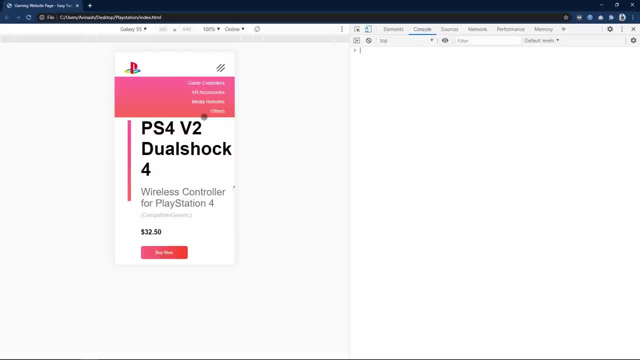 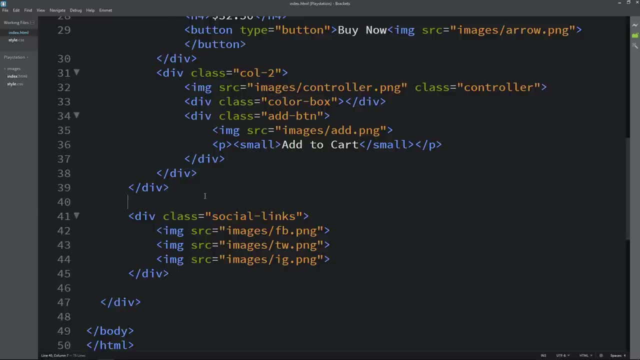 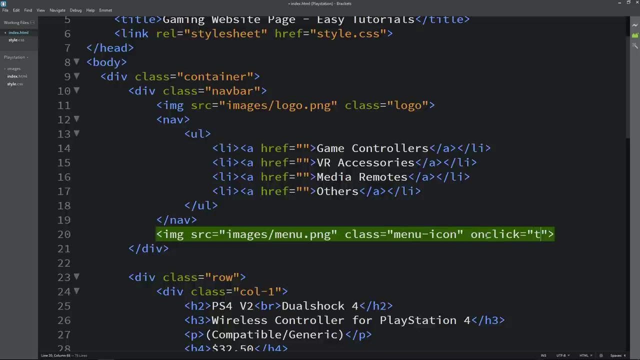 so next we have to add click event on this icon. so just come back in the HTML file and let me find where we have written the icon. so here it is. here we will add on: click on click equals toggle menu. so when we will click on this icon it will call the function. 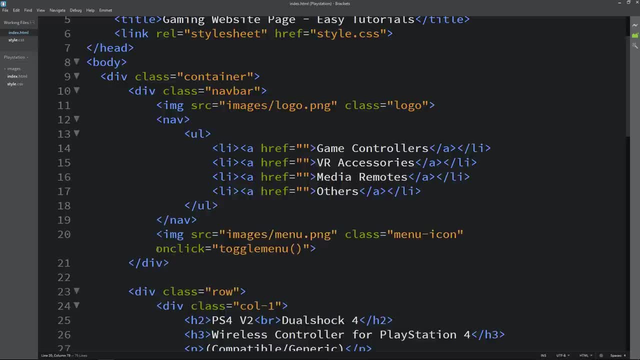 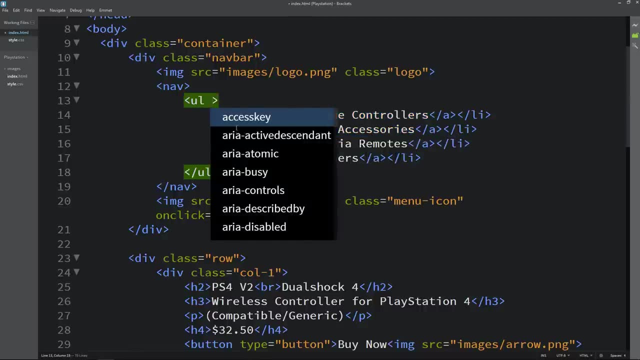 toggle menu. so we will create this function on the button click. we have to hide and display this list, which is in UL. so in this UL we will add one ID. so the ID am adding menu list. let's copy this one. Now come to the bottom. before this closing body tag here: 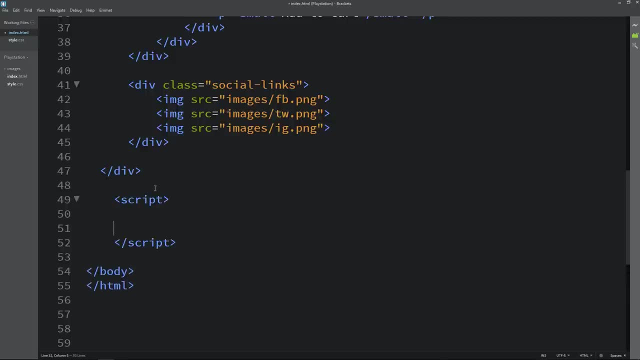 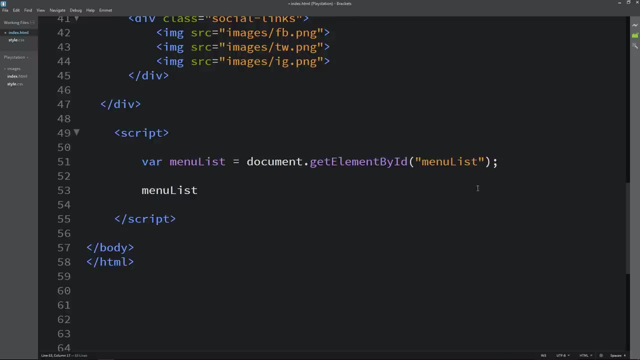 we will write a script open and closing tag. then write where menu list equals documentget element YID and the ID which is menu list. after that, here we will add menu list dot. style. dot max height equals zero pixel, so it will add zero pixel maximum height. next we will create the function with the name toggle menu. 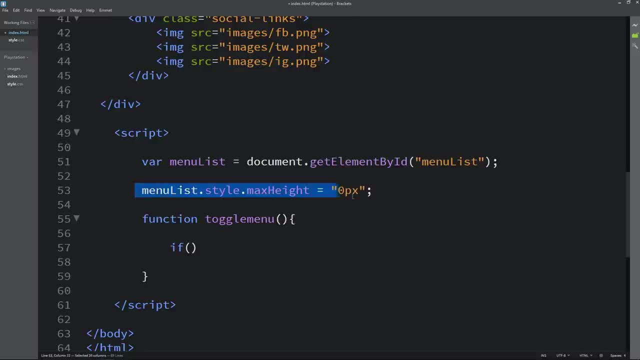 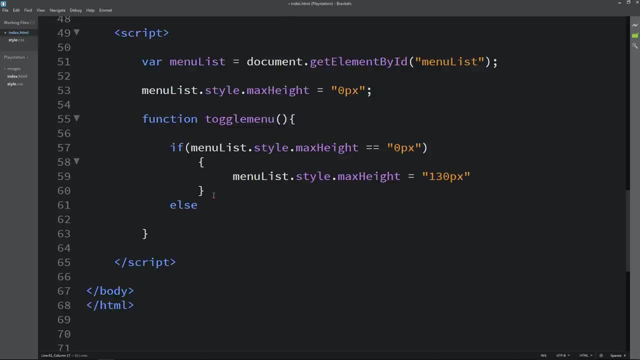 and in this function first we will check, if this one is equal to zero. for that here we will add double equals, so it will compare. after that we will write menu height dot style dot. max height equals 130 pixel. and here we will write else condition. in the else condition we will write: 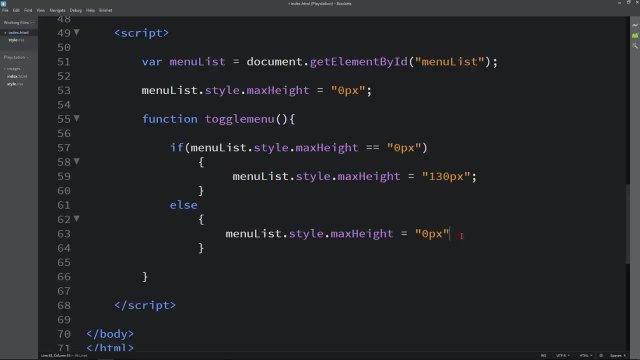 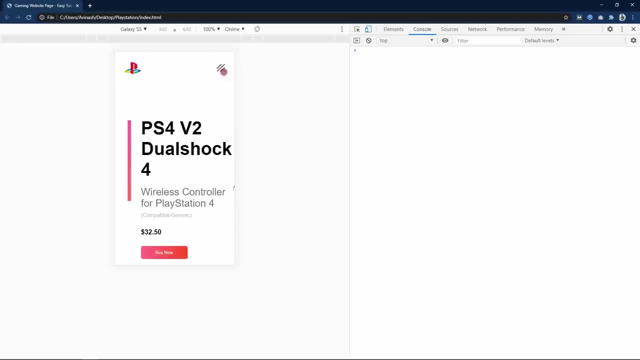 the same thing and it will be zero pixel. that's it. so now you can see if i click here it will display and hide this menu. but right now it is not very smooth for that. copy this id menu list and we will add menu list. dot. style: dot. max height equals one thirty pixel. 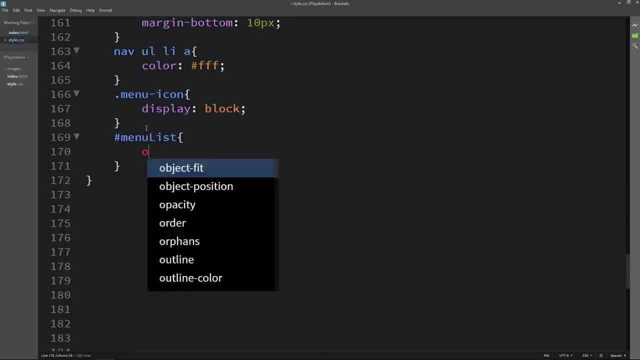 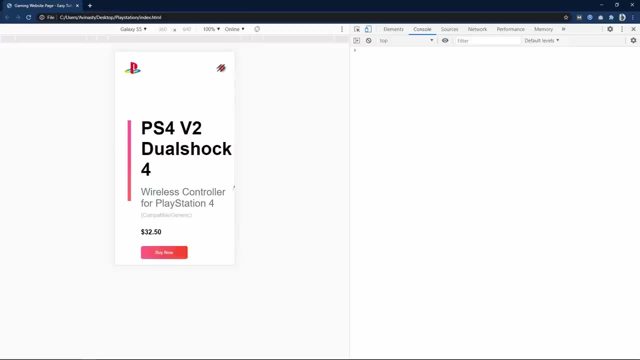 and come to the css file in the media query. here we will add menu list and overflow hidden and transition 0.5 second. that's it. after adding this, refresh the web page. and now, if i click on this icon, it will close and open this navigation menu very smoothly and right now you can see it. 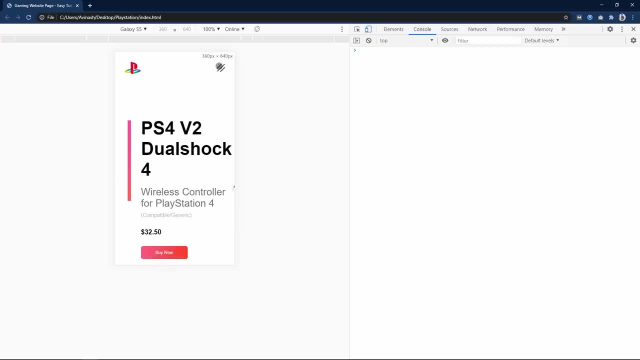 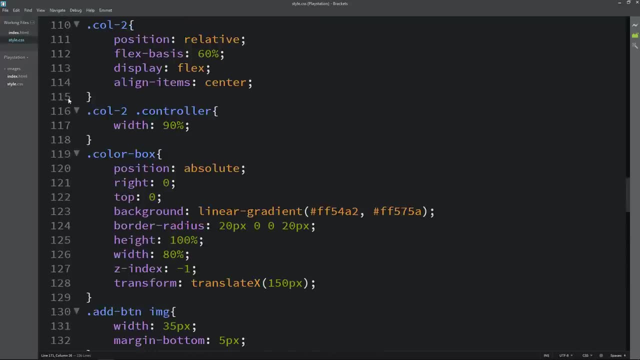 is coming like this: in the full screen and a small screen. it is coming like a toggle menu. next we will write the css properties for the other content on the web page. for that come back to the css file, and in this css file you can see we have added this row and here we have margin. 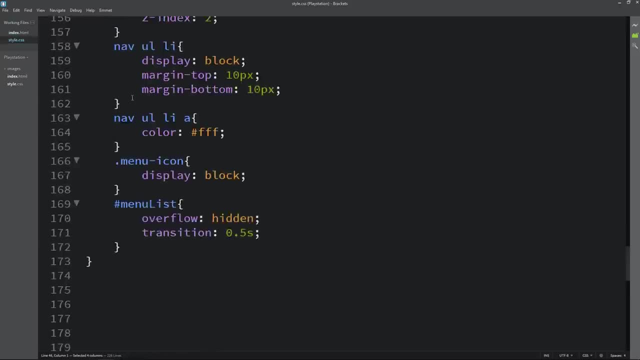 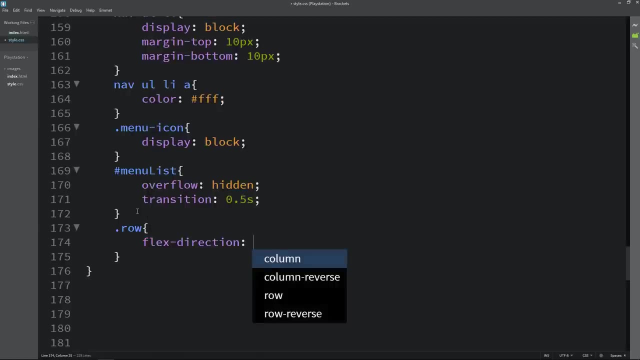 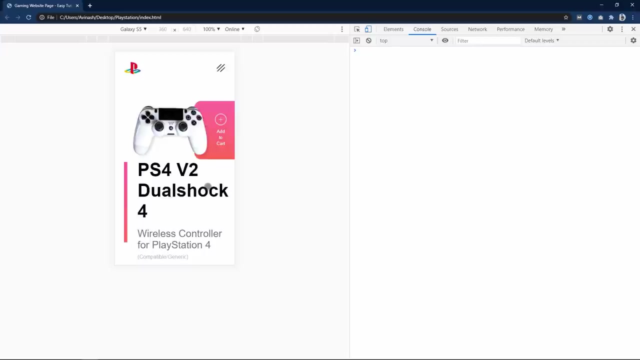 100 pixel and zero, so we will decrease this margin. so just copy this row and add it in the media query. here we will add flex, direction, column reverse and margin: 50 pixel, 0. after adding this, you can see this controller icon is also visual And we have less space from top and bottom. 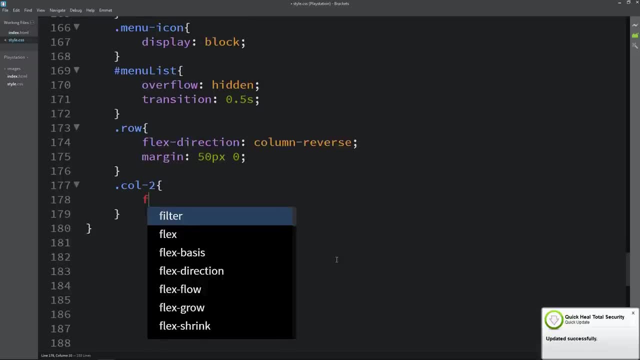 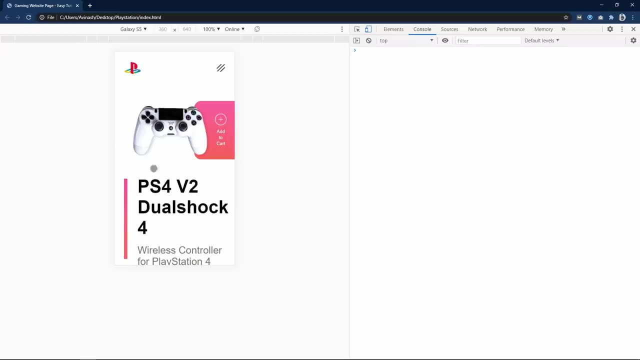 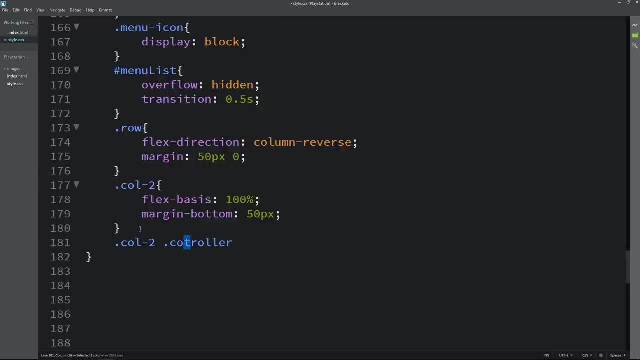 After that, here we will add call to and flex. basis it will be 100% and margin from the bottom. Now you can see some space from the bottom of this controller. Let's copy it again, then write controller and we will change the width. 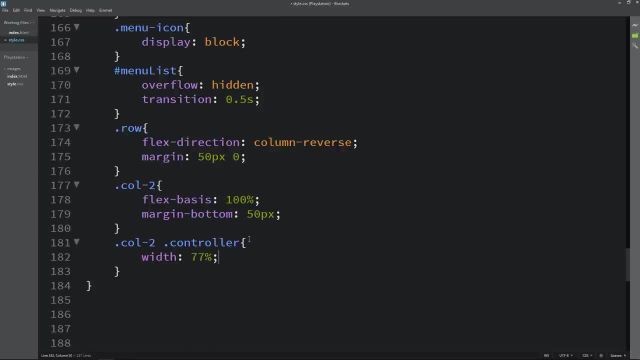 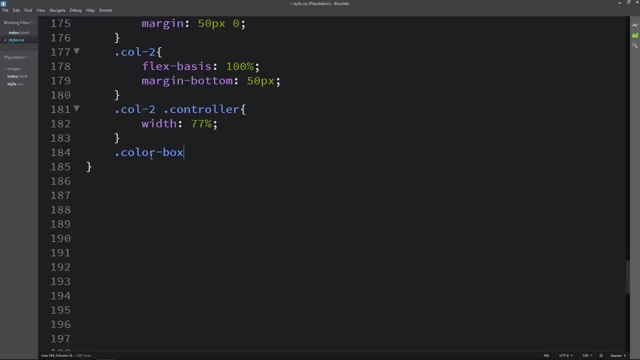 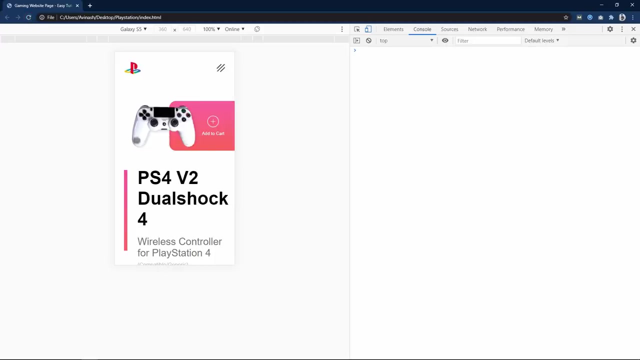 So here we will add width 77%. Now you can see different width. Now you can see we have this color box, So write it here in the media query and here we will add transform translate x 75px. After adding this, it is looking good. 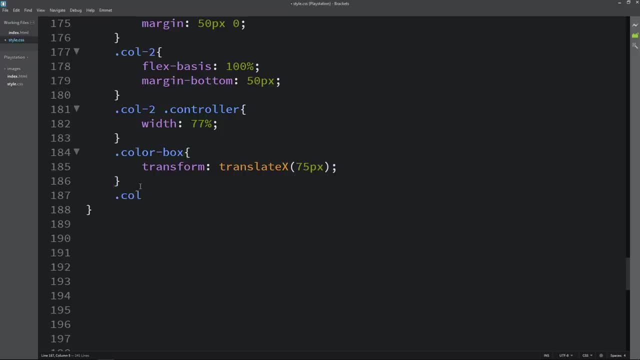 Next we will write the CSS properties for the other column. So just come back in the CSS file and here we will write call 1 and flex basis will be 100%. Again, copy this, then write h2 and we will decrease the font size so it will be 35px. 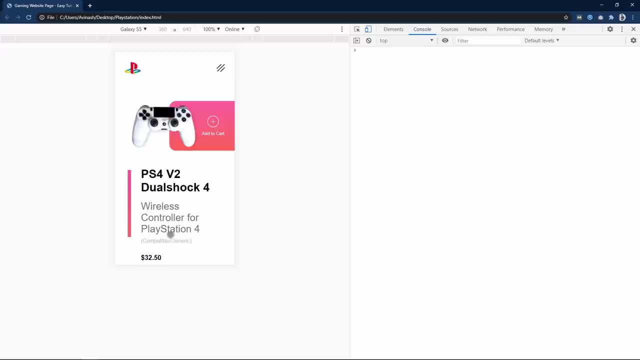 Now it is looking good. Let's decrease the font size for the other column. So just come back and duplicate this one, And here we will change it to h3 and it will be 15px. Now it is good. So now all the contents are looking good on this small screen device also. 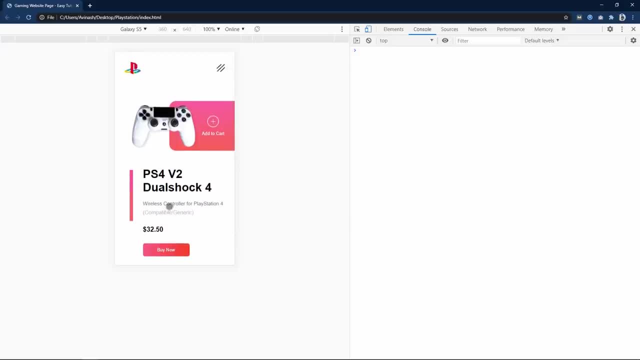 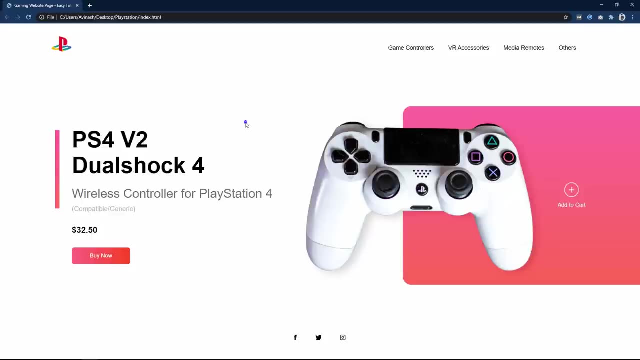 And this button hover is also working, And if I open this web page in full screen here also, it is looking very good. So this is how we have created this responsive web design using HTML and CSS and toggle menu using small javascript. I hope this video will help you.